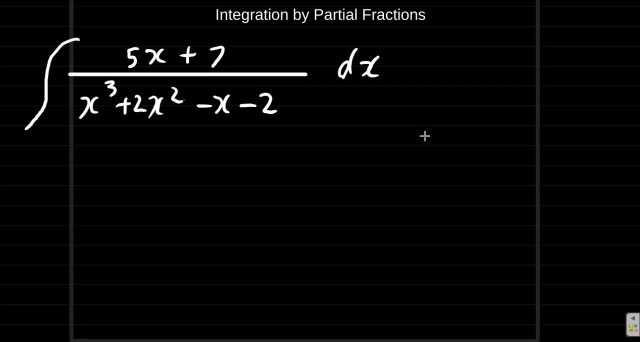 This is an example of an integration by partial fractions. This particular example is somewhat difficult, long and complicated. I hope that you will not get an example like this in exam, Maybe as a take home assignment or so, But not in a sit down exam. Now here you have X cubed plus 2X, squared minus X minus 2.. We want to find what the factors are for this. So let's put this aside: X cubed plus 2X squared minus X minus 2.. 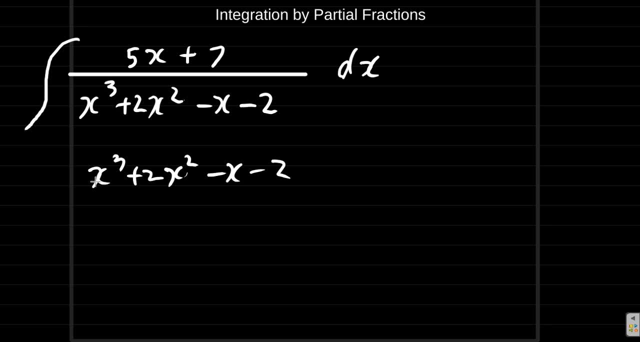 Now let's look at this. Suppose we consider the X cubed and the X squared here and factorize just these two alone, We have X and X squared plus 2X. Oh, we could take out X squared Right. X squared is the highest common factor, So inside the bracket we have X plus 2.. 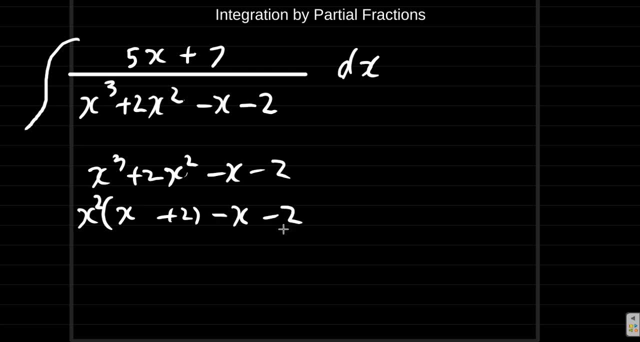 Minus X minus 2.. Alright, We have an X plus 2 in brackets. Suppose we put a bracket around this, We would have an X plus 2 in another bracket. So this is equal to X squared: X plus 2 minus minus open bracket: X plus 2.. See that. 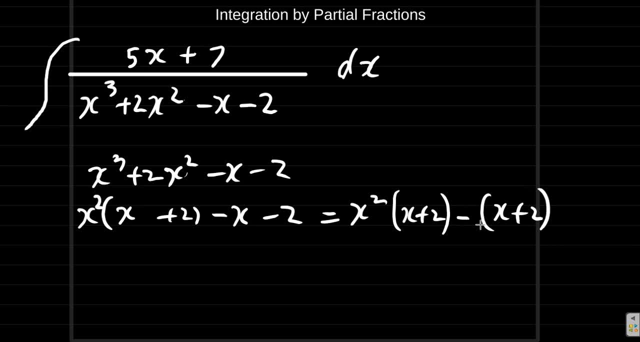 Alright, Now what is that equal to? Oh, we could factor out the X plus 2 as a common factor: X plus 2.. Because this X plus 2 here is a common factor here. So what you have inside the bracket is X squared X plus 2 times. this gives you X squared X plus 2.. So this is X squared. You have a minus sign. 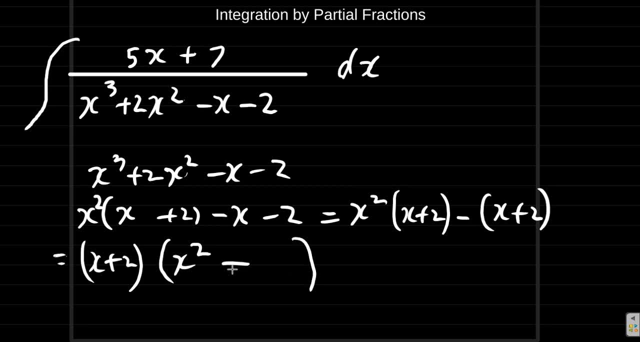 Minus before. Alright, Let's close the bracket and figure out what we're going to put here. X squared times: this will give us Now X plus 2 times. this will give us X plus 2.. It's going to be 1. Alright. 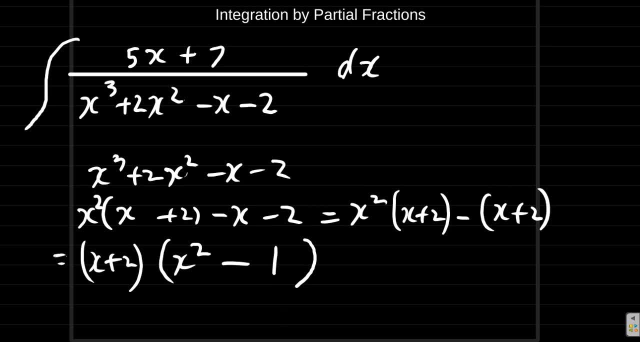 Now it could be factorized further, because notice that we have an X squared minus 1.. Which is a difference of 2 squares. So let's put back the X plus 2 here And then here The shortcut for factorizing this difference of 2 squares- We're going to have X plus 1.. X minus 1.. Remember your difference of 2 squares. 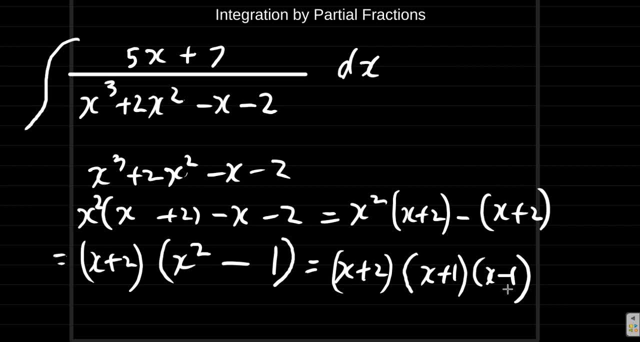 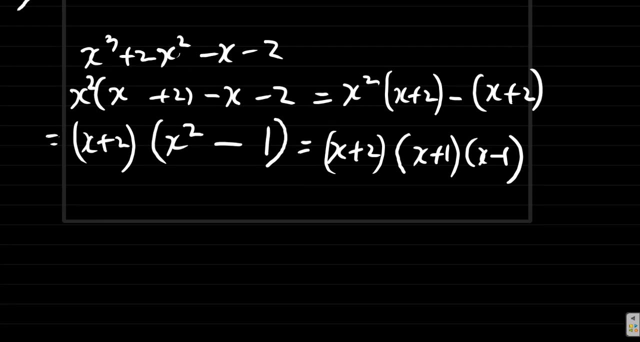 Alright, So that's what we have here. Alright, So We can write this thing as integral of 5X plus 7 over. So we have the integral of 5X plus 7 over X plus 2. X plus 1.. X minus 1. The X. 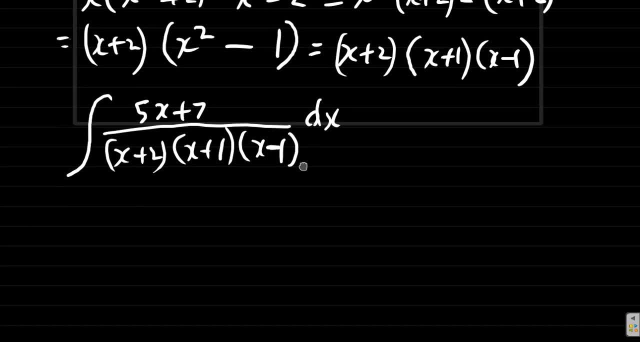 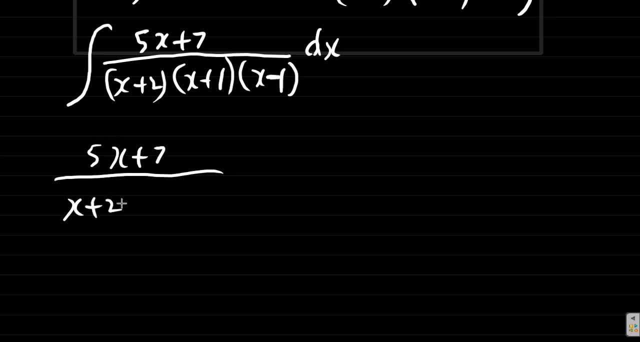 Now let's deal with the partial fractions, part. So 5X plus 7 over X plus 2.. X plus 1.. X minus 1. Is equal to. These are distinct linear factors. That means they are linear Right. The highest power of X is 1.. So it's X to the 1 in each. 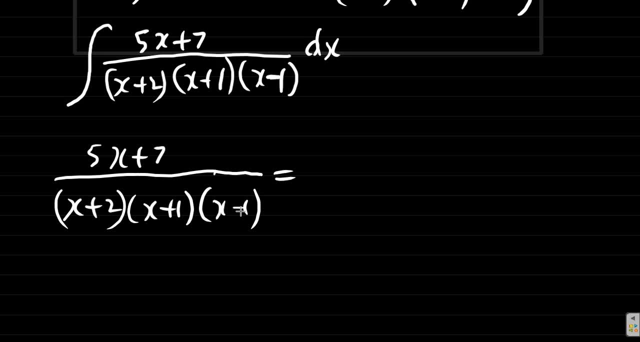 And they are distinct. They are different. So what you're going to have here is the farm A over X plus 2.. 2 plus b over x plus 1 plus c over x minus 1.. That's the form the partial fractions will. 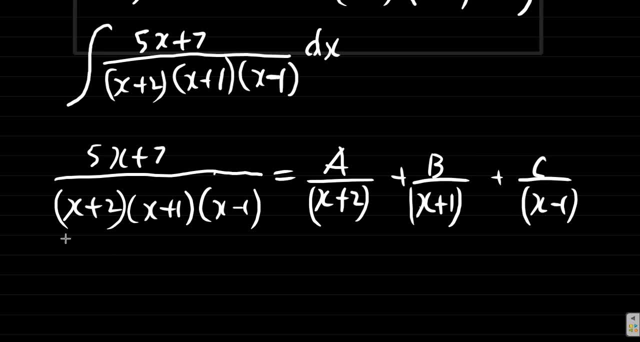 take. So what we have here now, what we're going to do is multiply by x plus 2, x plus 1, x minus 1.. See that That's what we're going to do When we multiply everything by x plus 2, x plus 1,. 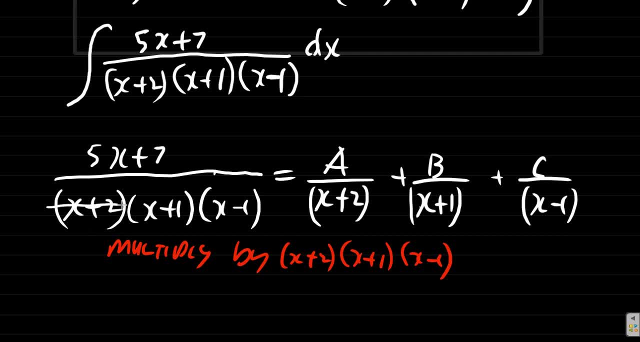 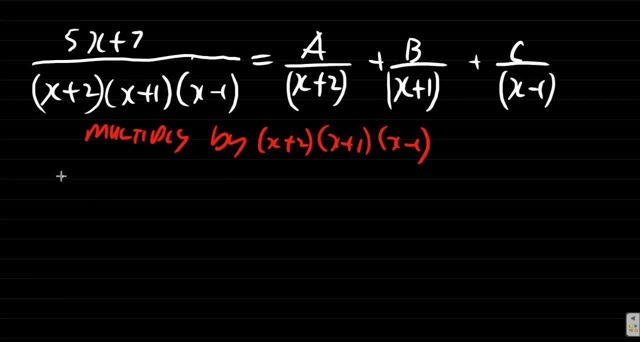 x minus 1,. all of this will cancel, See that, Because what we have is going to be 5x plus 7 over x plus 2, x plus 1, x minus 1 equals we have a over x plus 2. 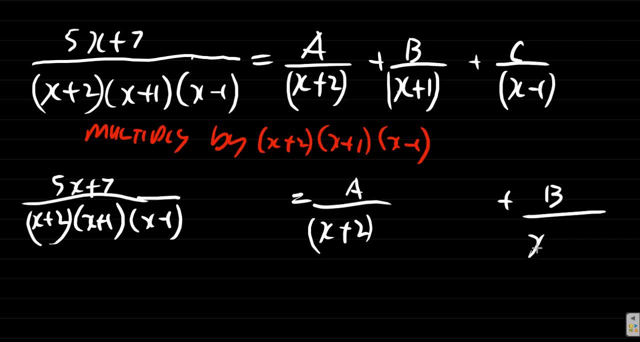 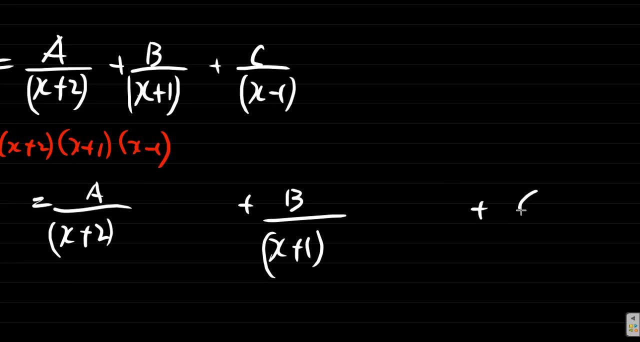 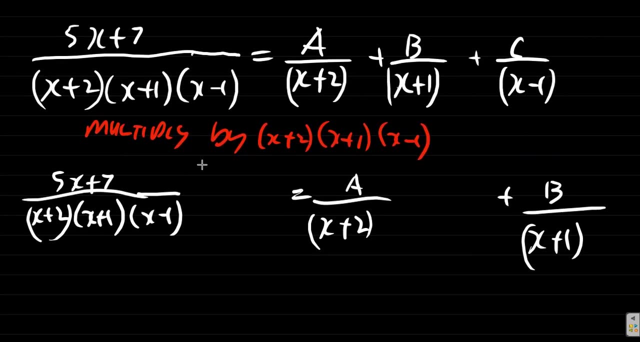 I'm putting some space between them: plus b over x plus 1, plus c over x minus 1.. So what's going to happen here? We multiply by x plus 2, x plus 1, x minus 1.. What happened: x plus 2- cancel x plus 2, x plus 1- cancel x plus 1.. 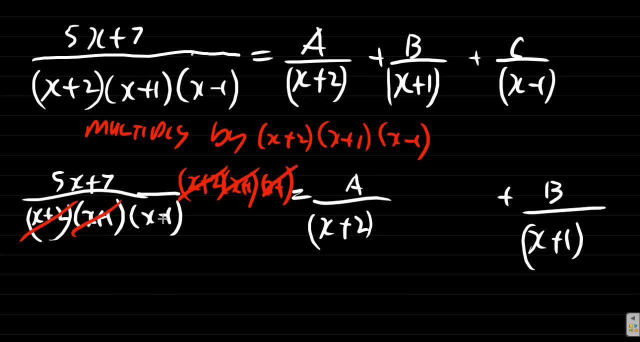 1, cancel x plus 1.. x minus 1, cancel x minus 1.. So you only will have 5x plus 7 here. Then you say equal. Then you multiply this by x plus 2, x plus 1, x minus 1.. x plus 2 will. 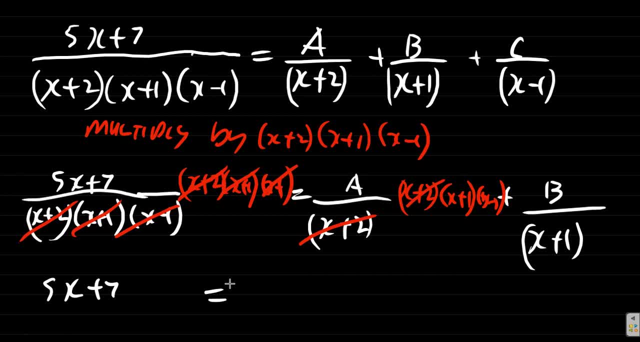 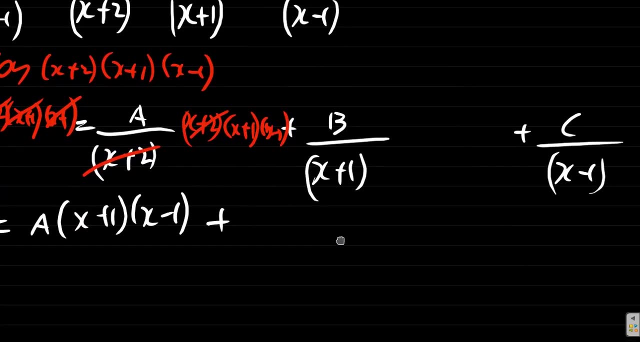 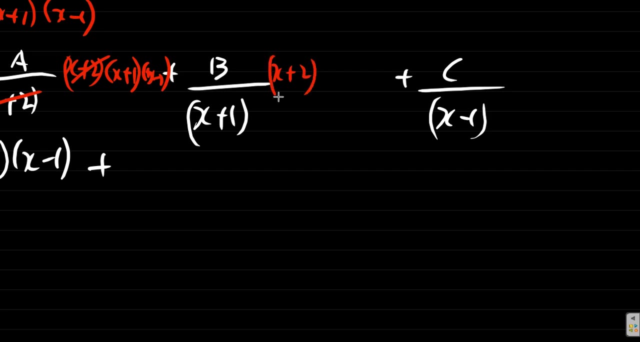 cancel x plus 2.. See that. So all you're left with here is ax plus 1, x minus 1.. See Plus. and then what's going to happen after that? My, my, this thing keeps jumping up and down. You're going to multiply this by x plus 2, x plus 1.. 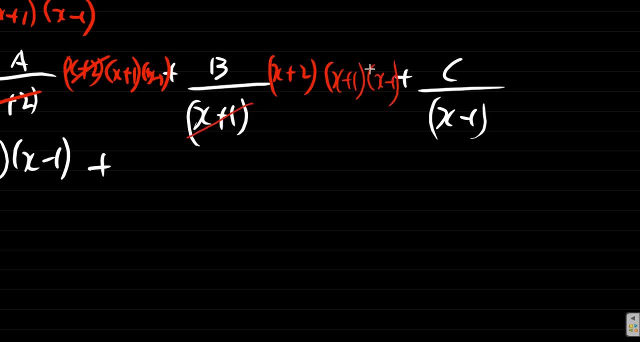 x minus 1, x plus 1 will cancel x plus 1.. So here you're left with b times: x plus 2, x minus 1.. See that, Plus What's going to happen out here now You have x plus 2, x. 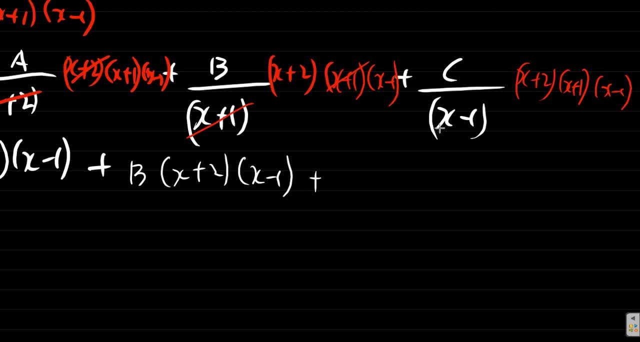 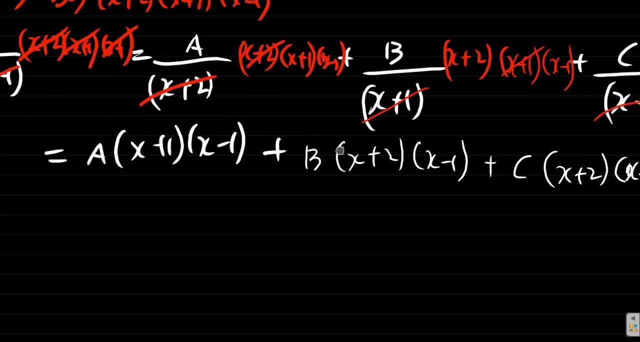 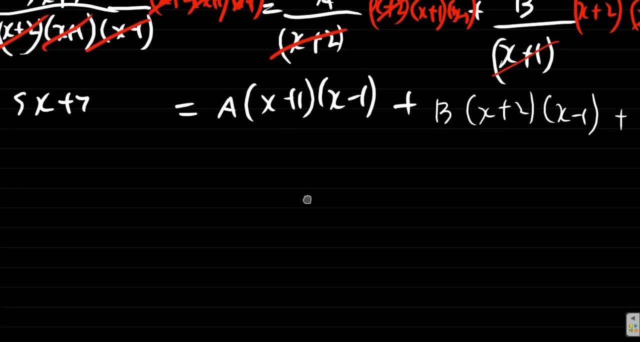 plus 1, x minus 1.. Multiply x minus 1 will cancel x minus 1.. So what you have left is C times X plus 2, X plus 1, right, So you have all of that. Now the next thing is going to multiply out the brackets. 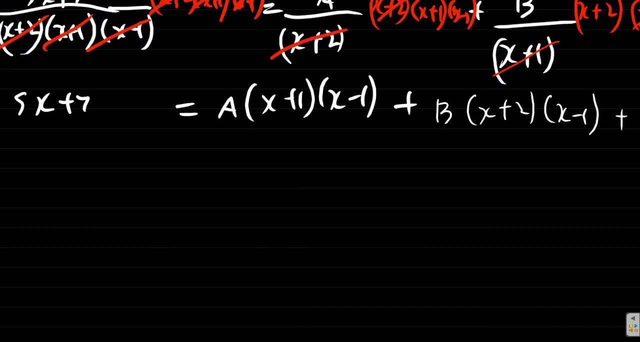 So we have 5X plus 7 is equal to 8 times. when you multiply out the brackets, you have X squared minus X plus X. that will disappear minus 1, right, Right Plus B times. you have X squared minus X plus 2X right. 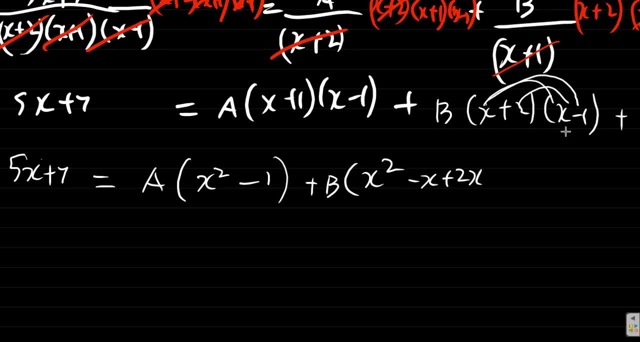 See X squared minus X plus 2X. But what's going to happen here? Negative X plus 2X, that's minus 1X. So you can't say plus X plus X, 2 times negative 1.. 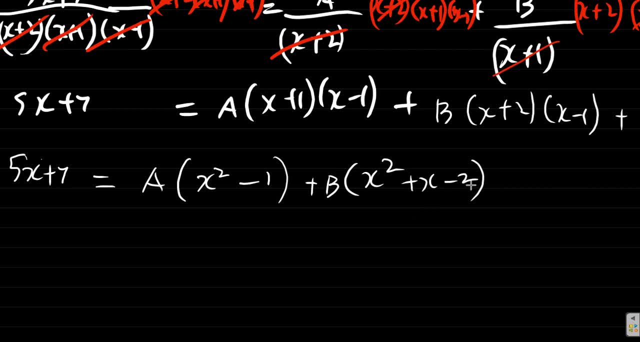 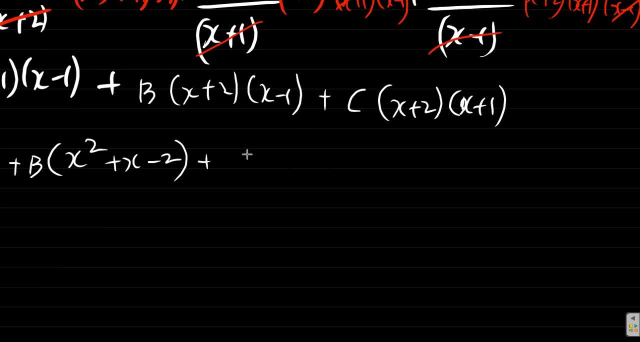 Minus 2, all right, So we have that Plus, And this is going to be C times X, squared plus 1X plus 2X, That's going to be plus 3X, 2 times 2 plus 2.. 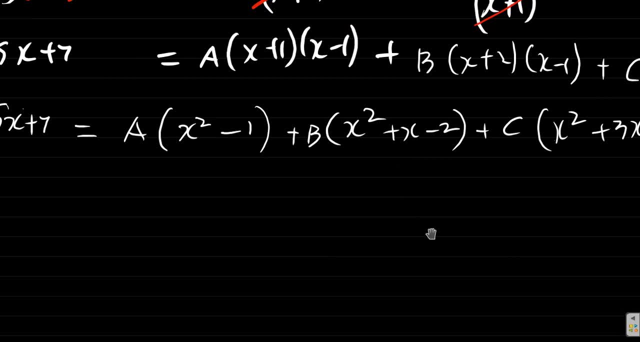 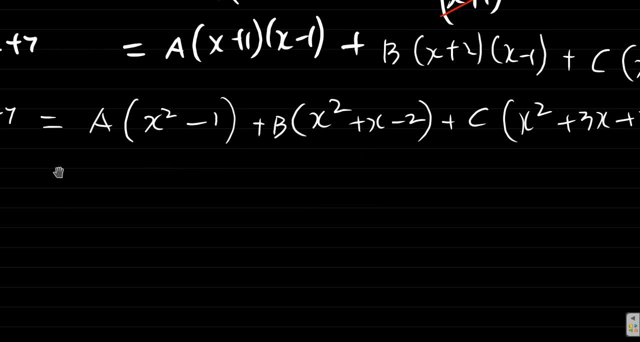 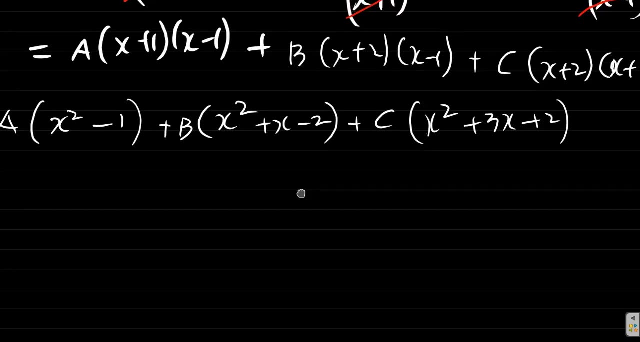 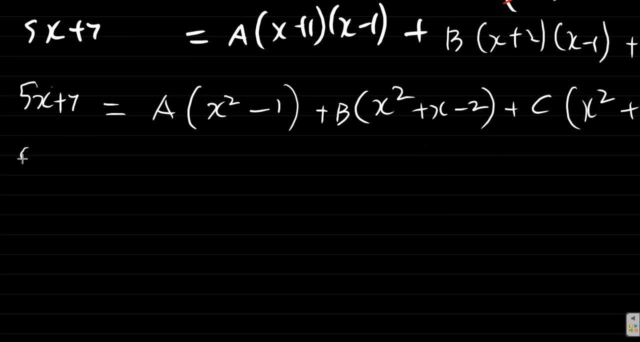 So there we have that. so far, Right, All right. So here let's expand the bracket and isolate the X squared, the X and the numbers. So what you have here is 5X plus 7 equals. you have AX. let me write it like this: AX squared. 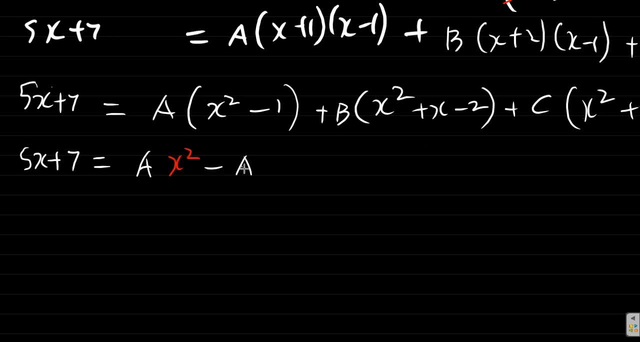 Right, Minus A plus BX. squared plus BX. We're going to write the X squared in red, The X is in blue. Then you say minus 2B, Minus 2B, Minus 2B. So these are the numbers. You have 2B. Write the numbers in yellow. Alright, And of course here this is 1A, So let me write 1A as well. Right, 1A. 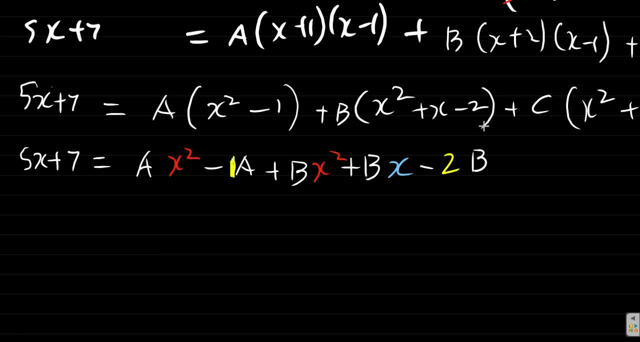 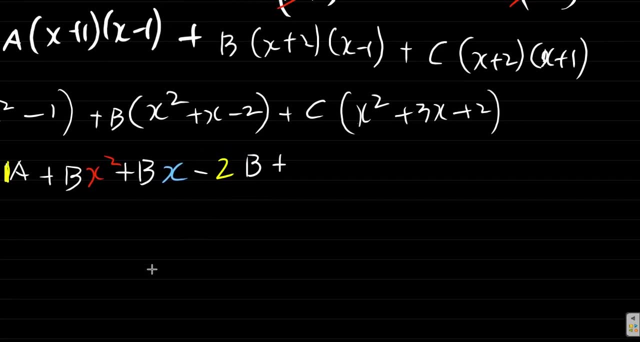 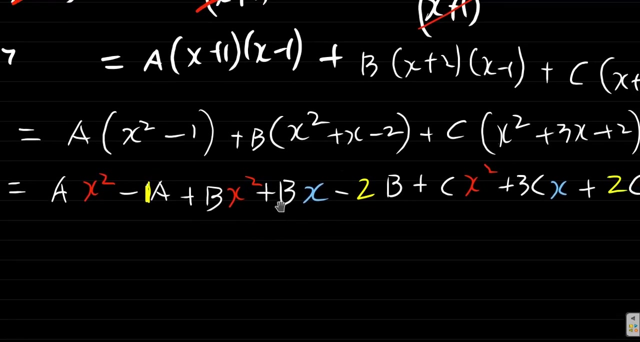 Then what happens after this Plus? Then you have CX squared, So you have CX squared plus 3CX, Right Alright, Plus 2. C- Alright. So here now we have AX squared minus 1A. 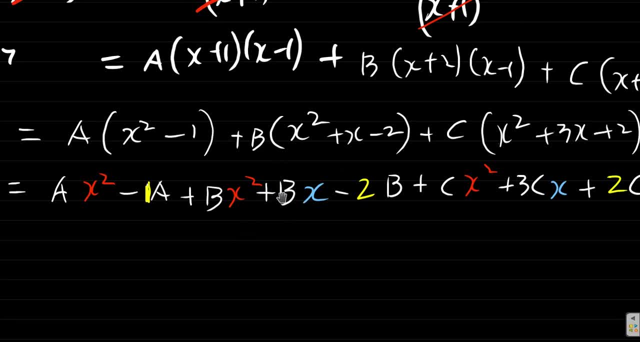 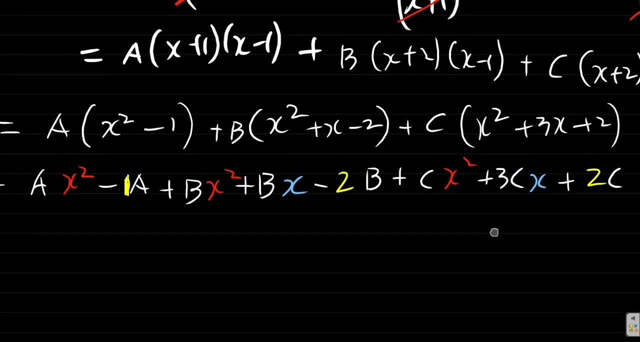 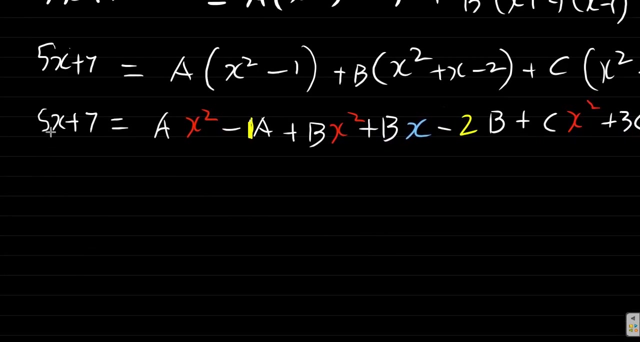 Plus BX squared plus BX minus 2B, Alright. Plus CX- BX squared plus 3CX plus 2C, Alright. So here now let's put like terms together: Now you have a 5X, So we have 5X plus you have a 7 there. 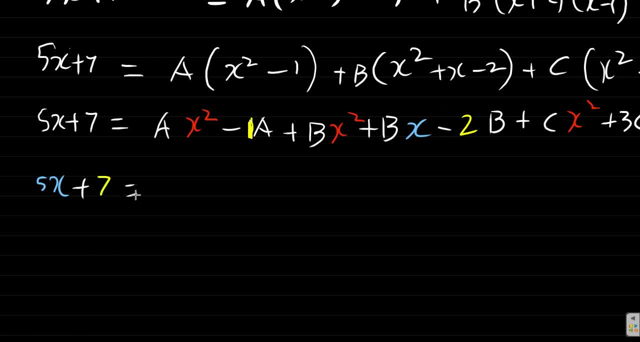 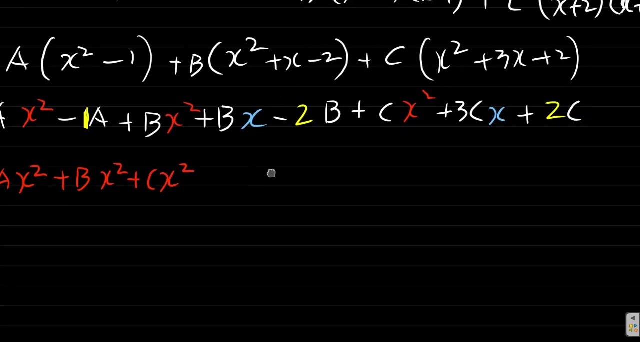 Let's put the numbers in yellow: Equal. Now the X squared parts. You have AX squared plus BX squared plus CX squared. Alright, You just want to separate them Not only by the X squared, but by the colors as well. You can see what's going on. 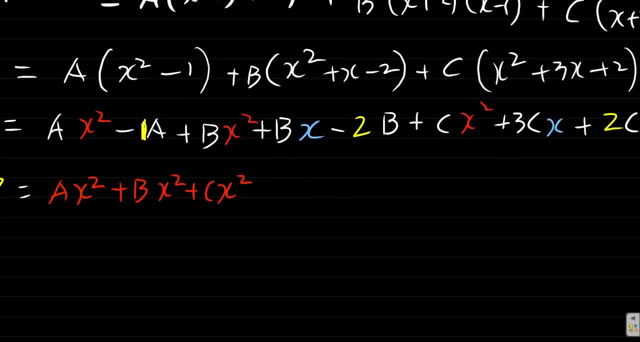 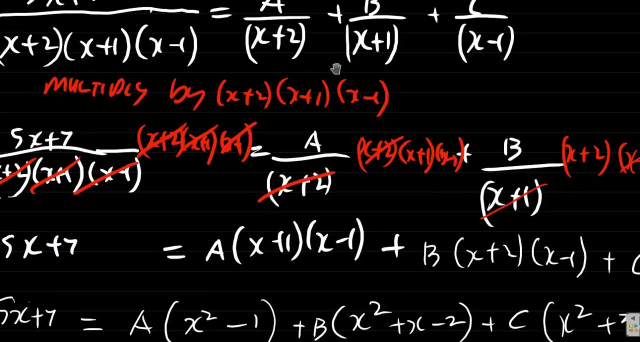 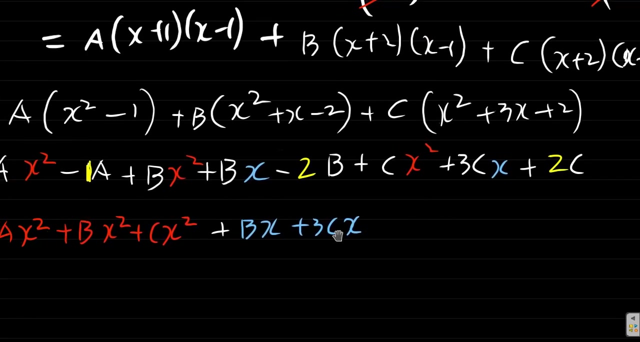 Then, after this, We have plus X's. now I want X's in blue. We have BX plus 3CX. Why this thing? jump all the way up there. No other X? Alright, No problem. Then the numbers now. 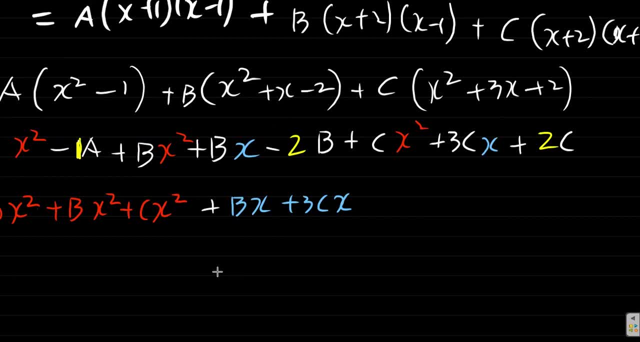 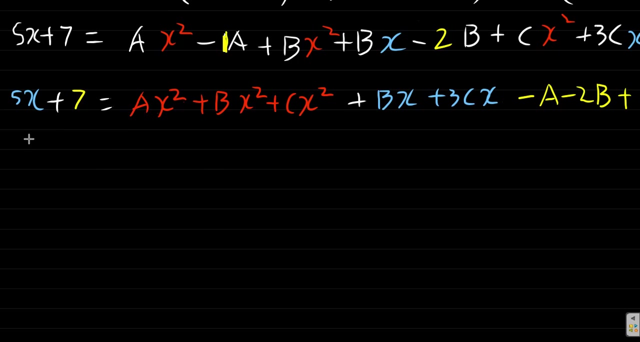 Then we have minus 1A, minus 2B plus 2C. Hopefully we accounted for everything, So what we have here It's 5X plus 2B. Alright, 5X plus 7 equals. 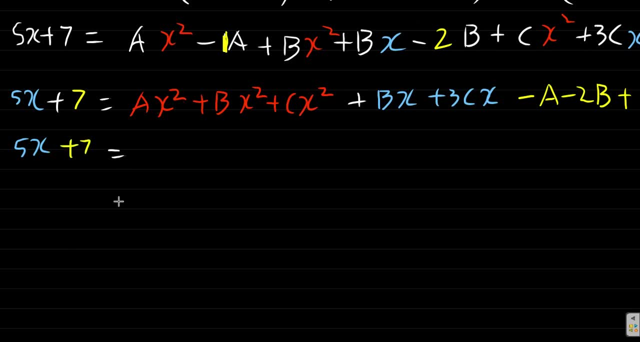 Let's put X squared outside the bracket. Let's put X squared. Times four times A plus B plus C. as an operator, I told you before I knew that this was a lot of work. Alright, Hopefully they don't give this to you in an exam. 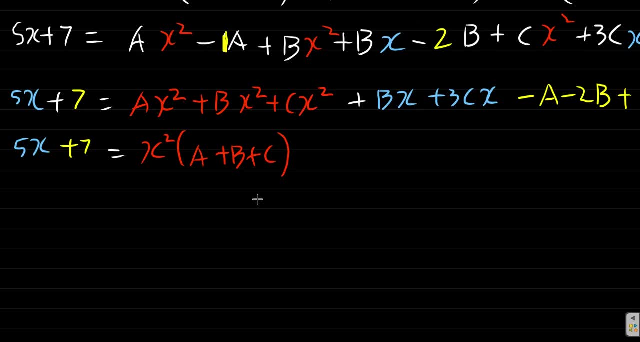 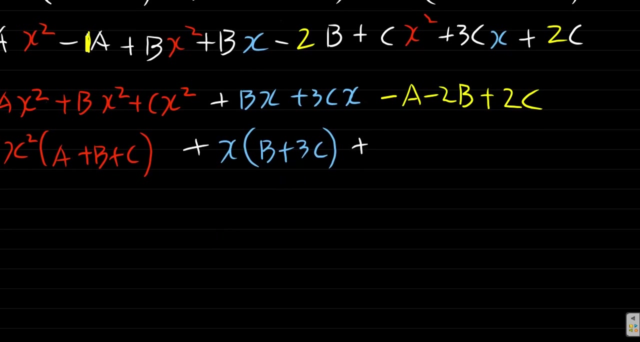 Well, maybe you get it, But you'll have enough time to work it out. you're compensated with a lot of marks, right? plus we have X, and then B plus 3 C, then we have here plus, then we have here: call it negative: a minus 2, B plus 2 C, all right, so 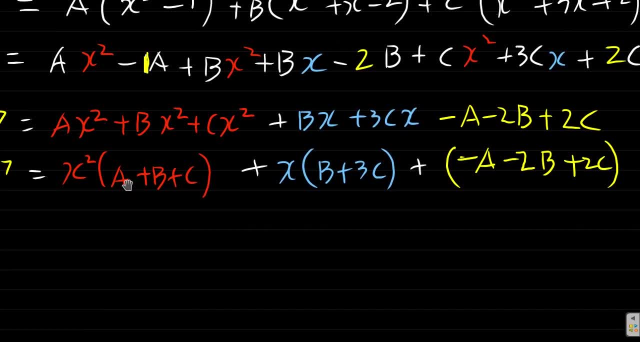 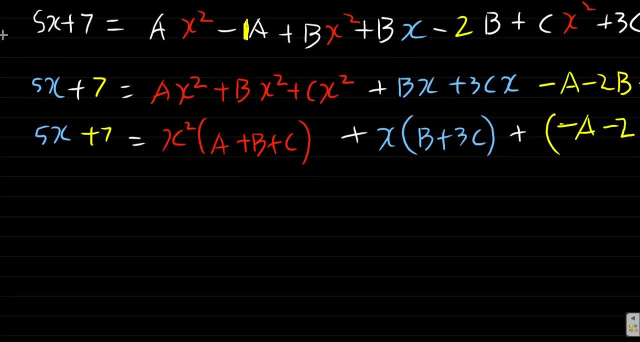 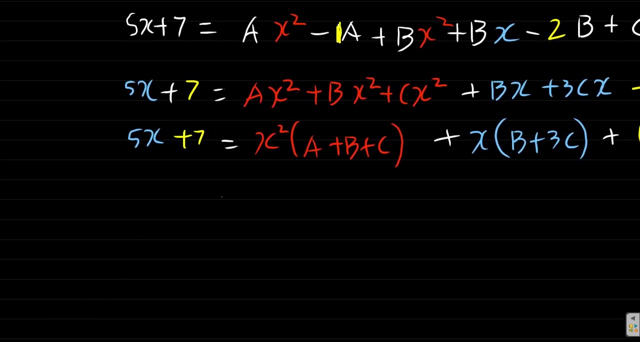 that's what we have at this point. all right, so let's equate what we have on the left and on the right. we see here that x squared can be written on the left as 0x squared. so comparing x squared and x squared, we can say that a plus B plus C is equal to 0. see that 0. this left and right are. 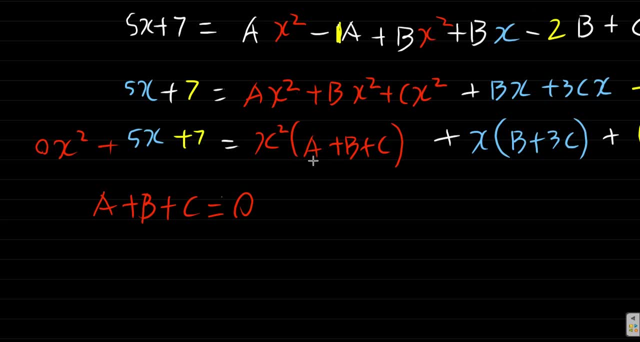 equal. so 0 times x squared is equal to a plus B plus C times x squared, a plus B plus P must be 0. then here, 5 times X is the same as B plus 3 C times X. so that means b plus 3 C must be equal to 5 and then 7. 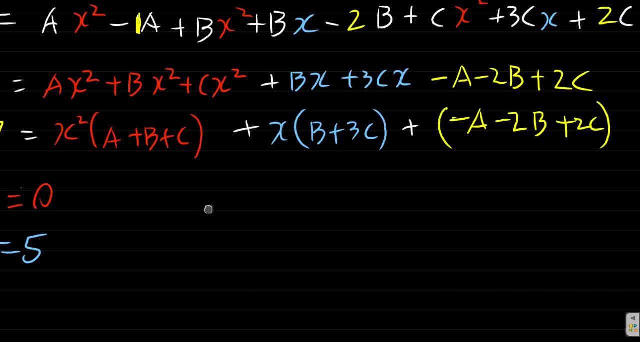 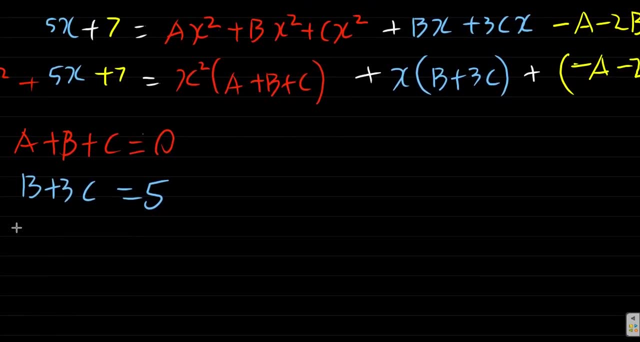 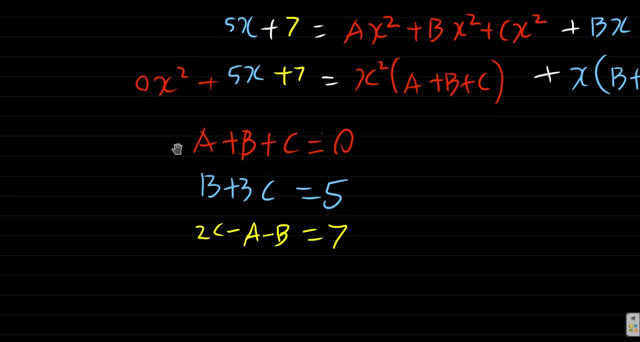 is equal to- lets put this positive one first- 2C minus a minus b. so we have 2C minus a minus b is equal to 7.. Well, we have three simultaneous equations to solve. now let's see what we can do with this. suppose we have this as equation one. equation two: equation three: 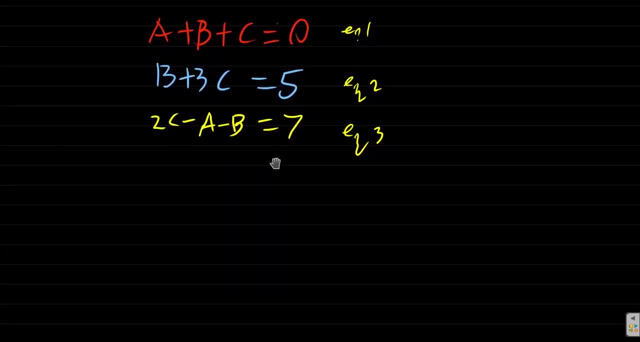 b. we can use what they call guardian elimination method to work this out. suppose we multiply, say equation two, no, equation one, multiply by three. so we would have 3b. it's writing right why 3b plus this would be: oh, this equation one, i'm multiplying, multiplying equation one by three. 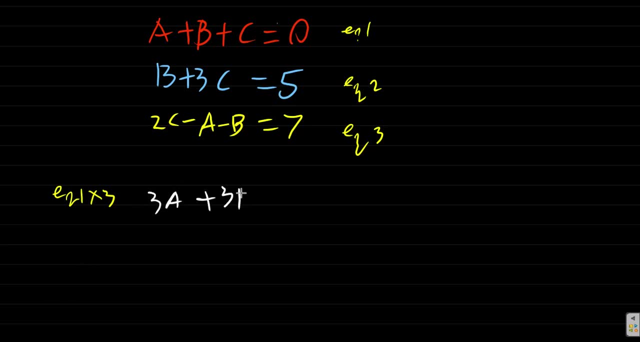 we would have three a plus three b plus three c equals zero. and then we put back equation two b plus three c equals zero. and then remember, this is equation two. and then we subtract: three a minus zero, is three a plus three b minus b. this two b equals zero. see that? so we eliminated c now. 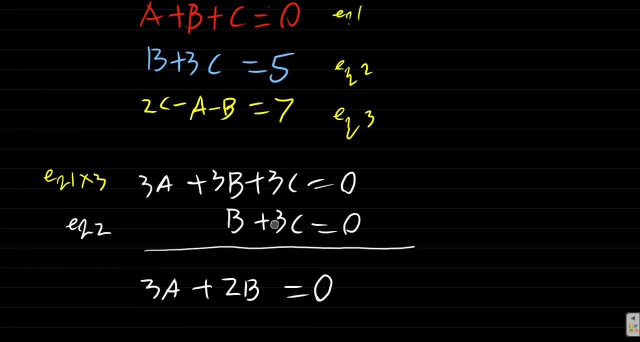 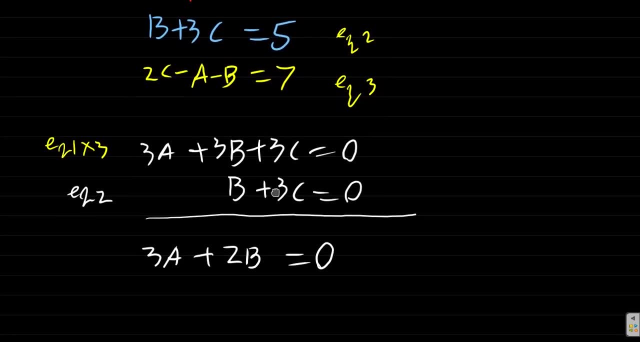 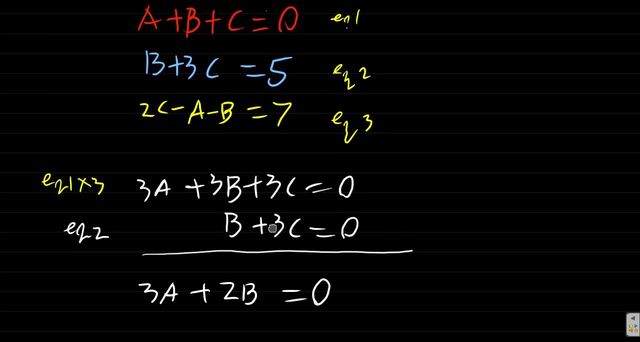 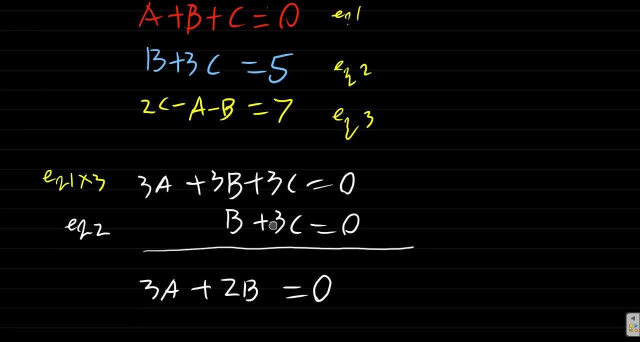 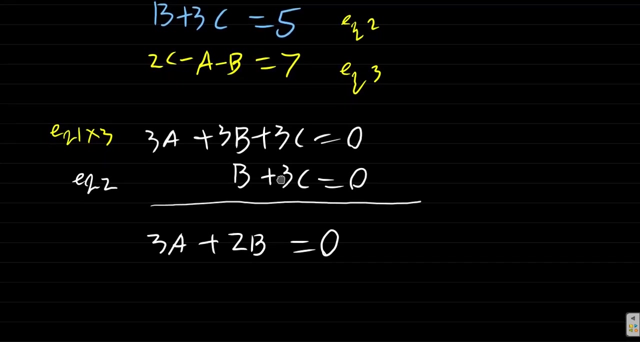 let's consider equation human. uh, let me see now equation three. suppose we multiply equation three by by what? now? by two? equation three multiplied by now by two. so this is a simple strategy: Equation 3 multiplied by 2.. So let's try another strategy. 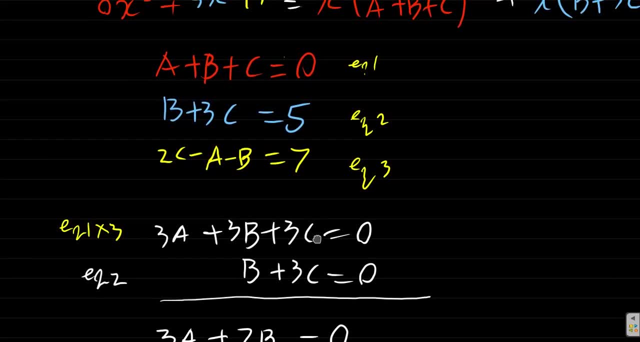 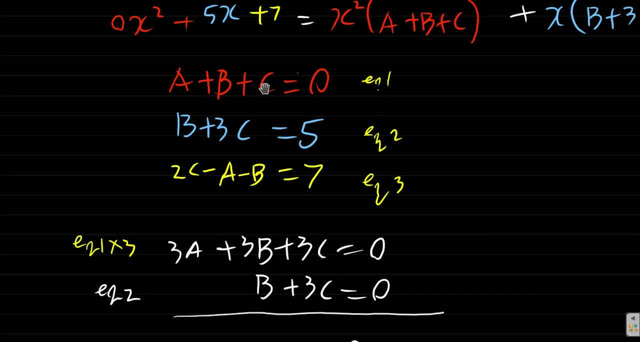 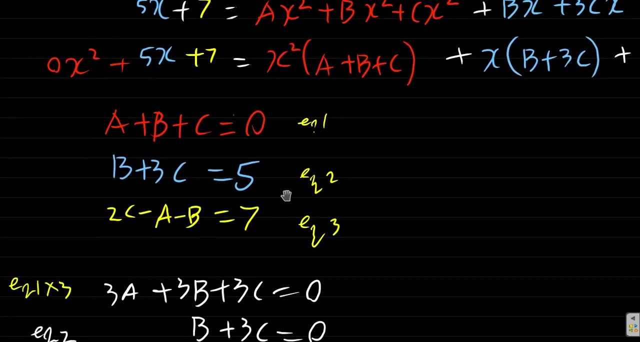 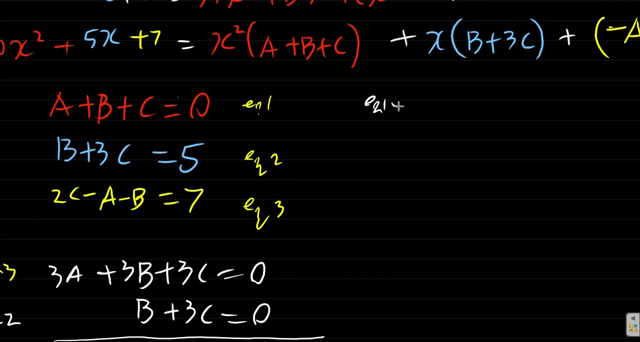 Oh Yeah, Equation 1 times 2.. Suppose we multiply equation 1 times 2. We'll get a 2C, And then we could eliminate the C Right. So we have equation 1 times 2.. Equation 1 times 2.. 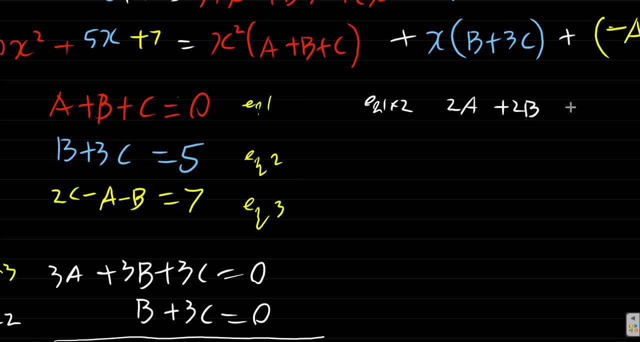 We have 2A plus 2B plus 2C equals 0.. Let's write back equation 3.. Let's put them in order: Negative: A minus B Plus 2C equals 7.. See that This is equation 3, you know. 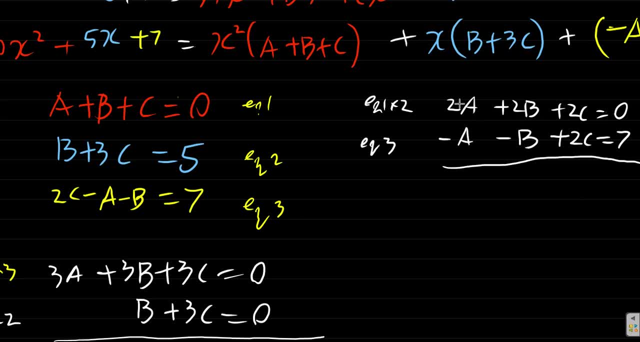 And then Suppose we subtract 2A minus negative, A is 3A, Then 2B minus negative B is 3B. 2C minus 2C, that's 0.. And then 0 minus 7 is negative 7.. 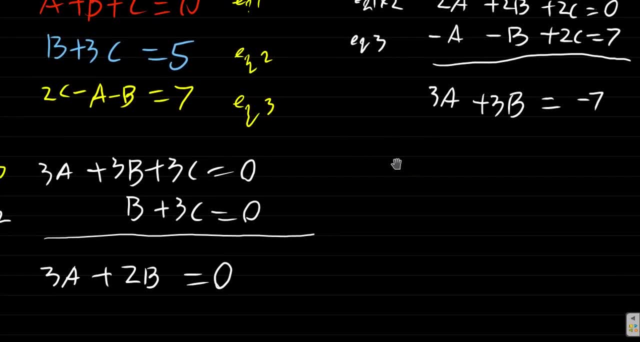 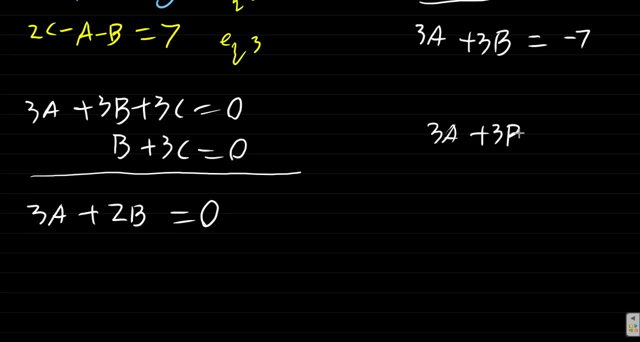 So what we have here are two equations in two unknowns. So we could solve for A and B. So here let's put them together: 3A plus 3B equals negative 7.. 3A plus 2B equals 0.. 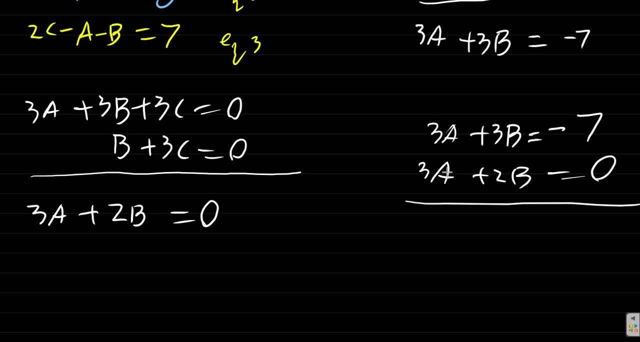 If we subtract these 3 to 3A minus 3A, that's gone. 3B minus 2B is B equals 7 minus 0. Negative 7 minus 0 is negative 7. So we see that B is negative 7.. 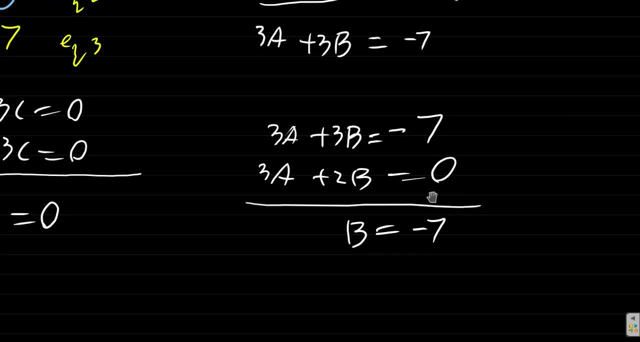 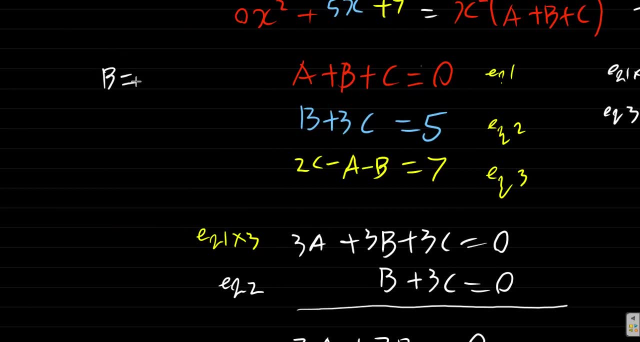 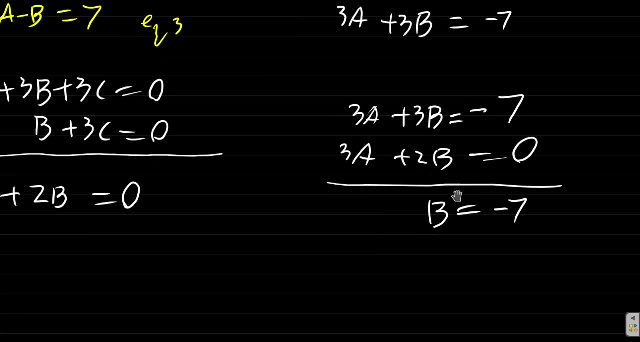 Alright, Alright, B is negative 7.. So let's write that up here: B is equal to negative 7.. Alright, I'm not able to scroll down any further. I've run out of space, But let's continue working. 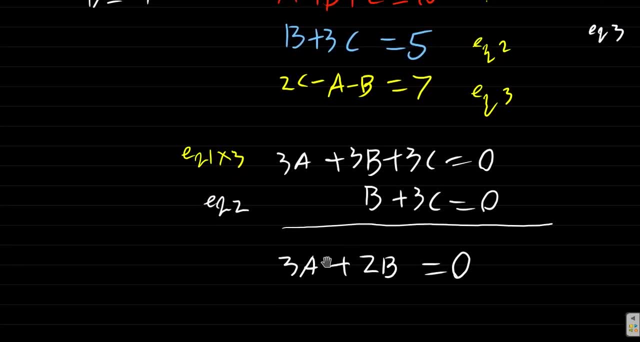 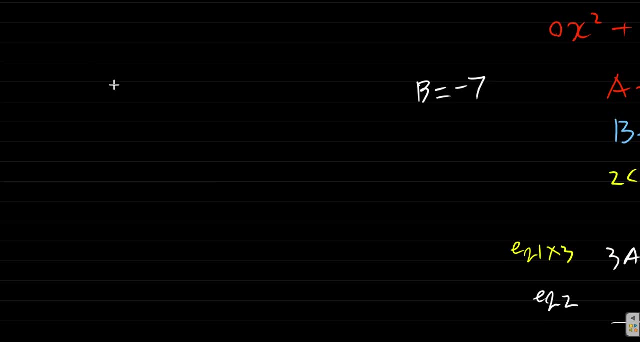 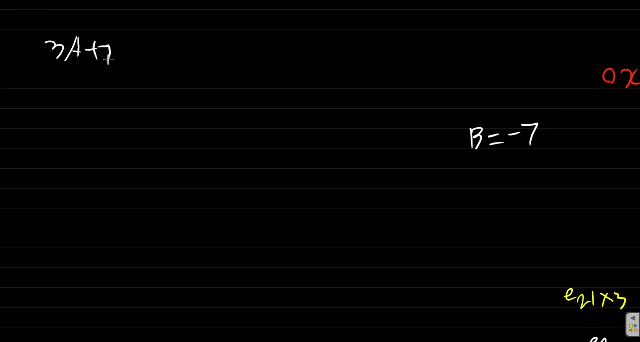 B is negative 7.. Now here, 3A plus 2B is 0. So let's work with that. So 3A plus 2B equals 0.. So 3A plus 2B. 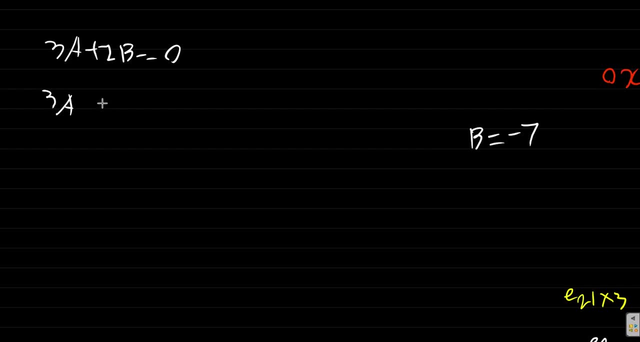 equals 0. That means 3A plus 2 times negative 7 equals 0. So 3A minus 40 equals 0. Alright, So that means 3A is equal to 14.. So A would be. 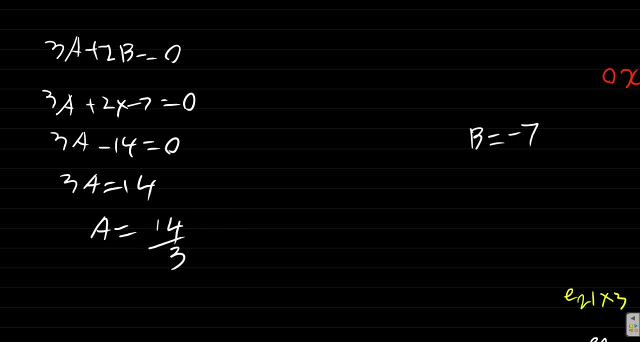 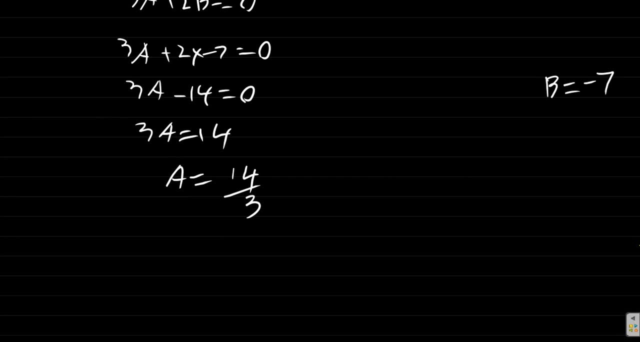 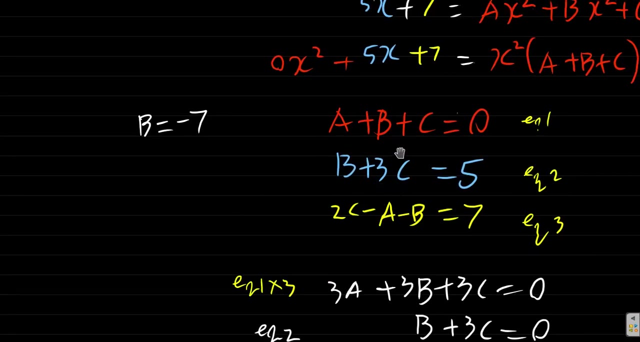 14 over 3.. Alright, So A is 14 over 3.. So we know that B is negative 7.. B is equal to negative 7.. And then let's use the equation 1, A plus B plus C equals 0.. 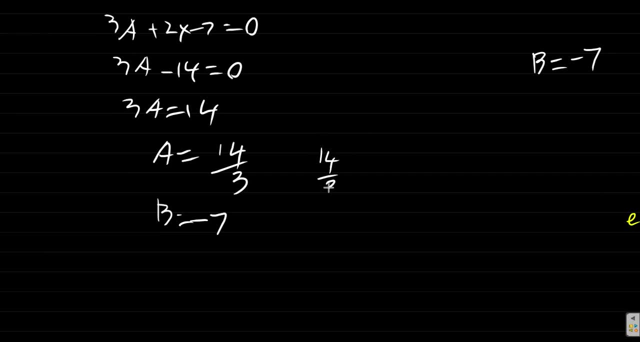 And see what it comes out to be: A, which is 14 over 3,, plus B, which is negative, 7, plus C is equal to 0. So now this is the same as 14 over 3 minus. 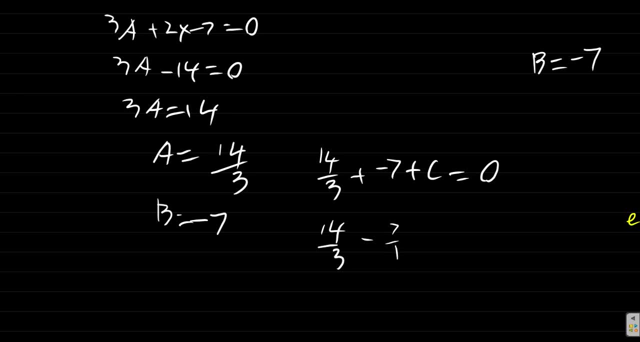 7 over 1, which is the same. 7 over 3 is 21.. So it's 21 over 3. using common denominators, This is 21 over 3 plus C equals 0.. So 14 minus 21. 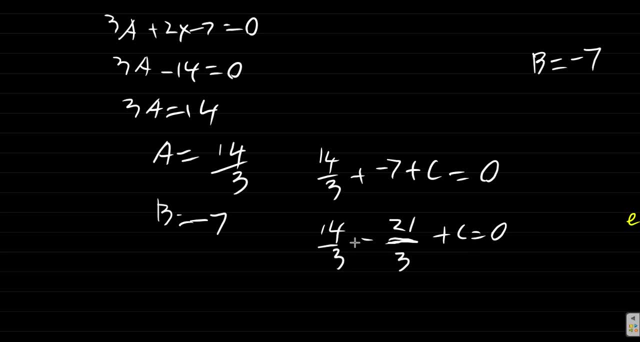 is going to be what? Negative 7 over 3. Negative 7 over 3 equals negative C. So C is equal to negative 7 over 3. C equals negative 7 over 3.. Alright, So that's what we have working with. 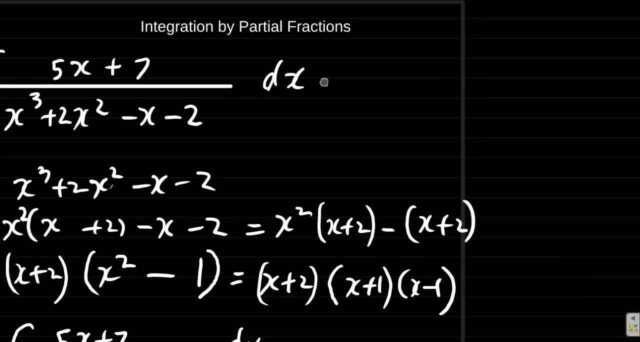 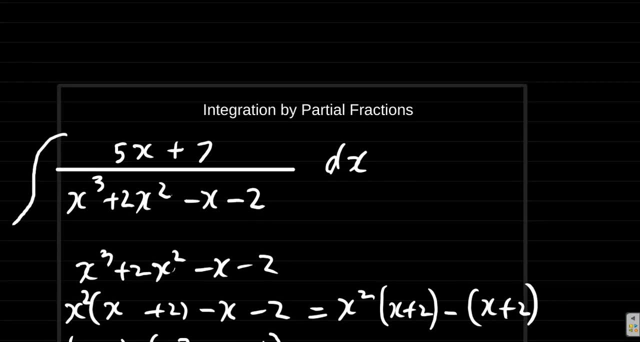 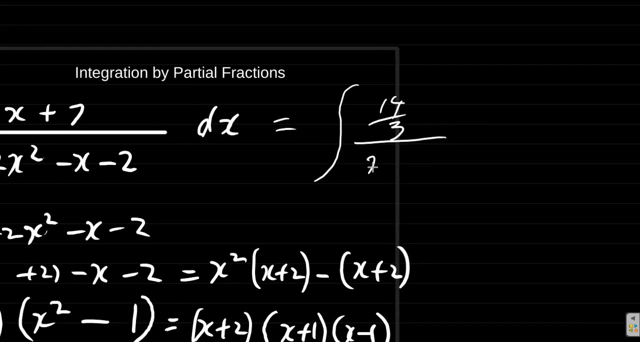 A is 14 over 3.. So let's scroll back up here So this can be written as the integral of 14 over 3 over, and it was A over X plus 2.. So it's X plus 2.. 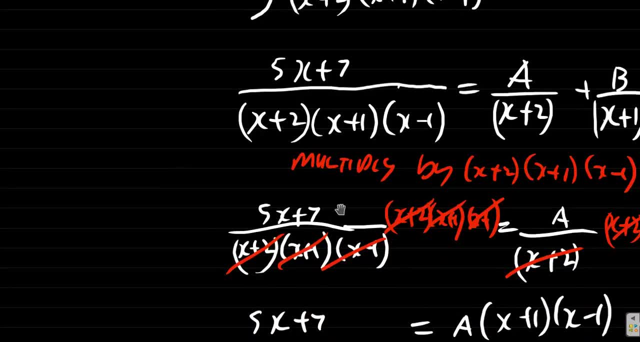 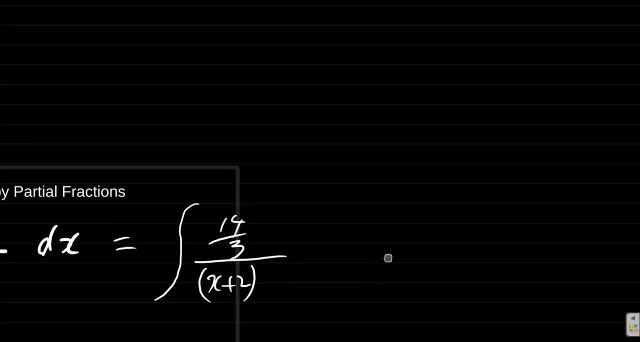 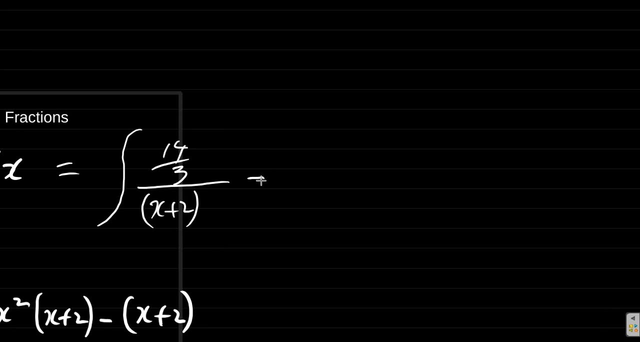 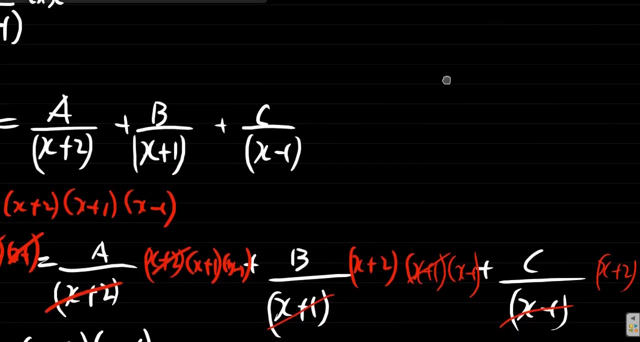 Alright, What was B? again? B negative 7. So we have negative 7 over X plus 1.. So we have minus 7 over X plus 1.. And then we look back at C. C is negative, 7 over 3.. 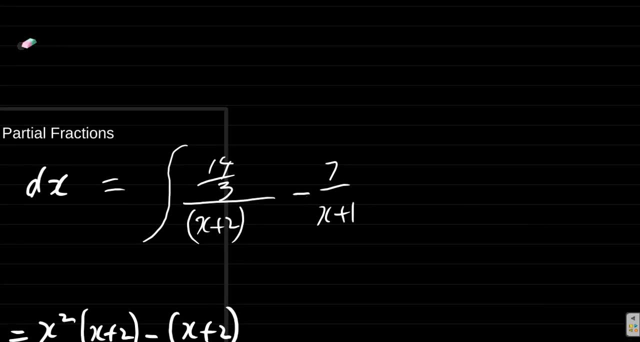 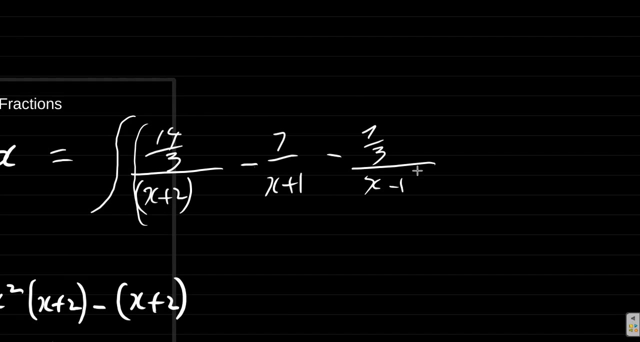 So we have- it is negative- 7 over 3 over X minus 1.. Alright, It's the same as now. if we integrate them individually, We have the integral of 14.. Well, we could put the 14 over 3 outside.